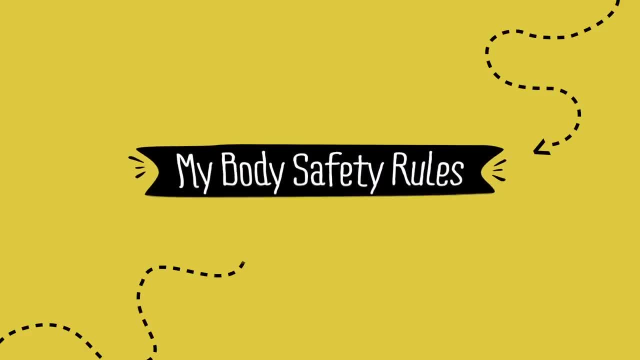 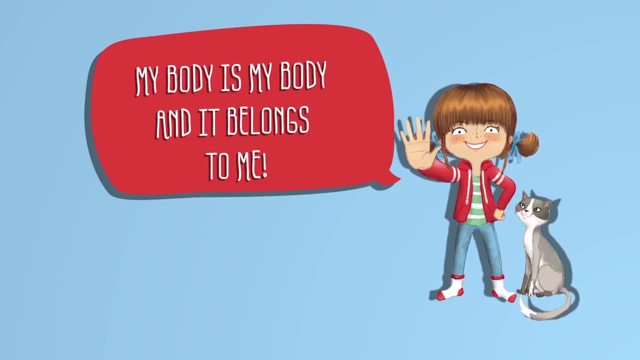 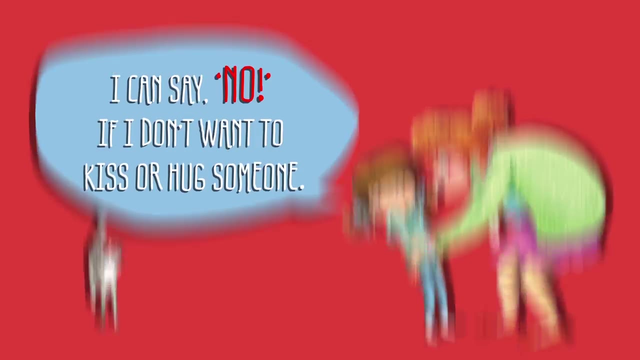 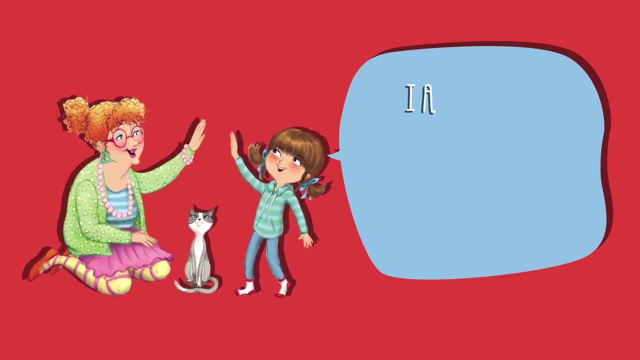 My body's safety rules. 1. My body is my body and it belongs to me. I can say no if I don't want to kiss or hug someone. I can give them a high five, shake their hand or blow them a kiss. I am the boss of my body and what I say goes. 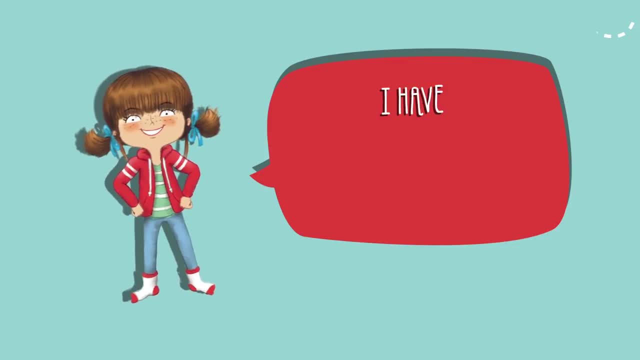 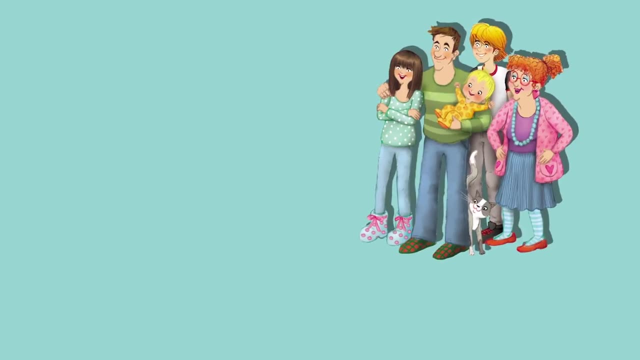 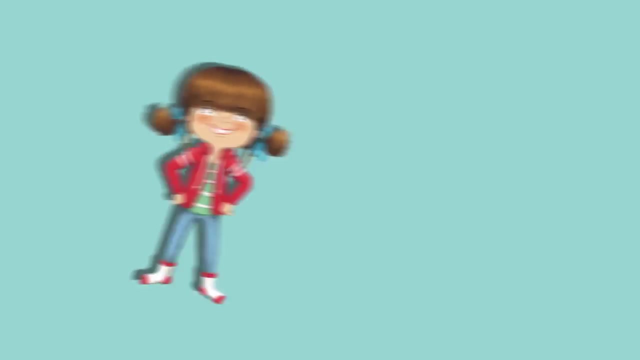 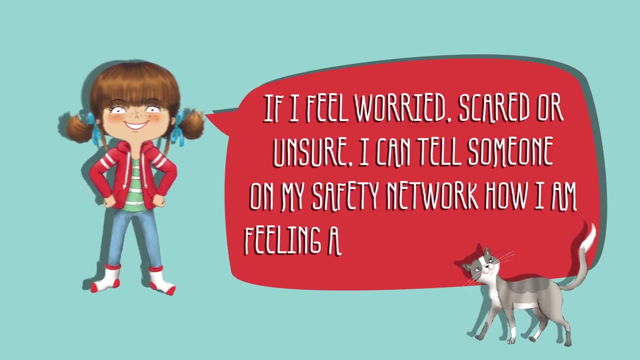 2. I have a safety network. Every person's safety network will be different. These are the adults I trust. I can tell these people anything and they will believe me. If I feel worried, scared or unsure, I can tell someone on my safety network how I am feeling and why I feel this way. 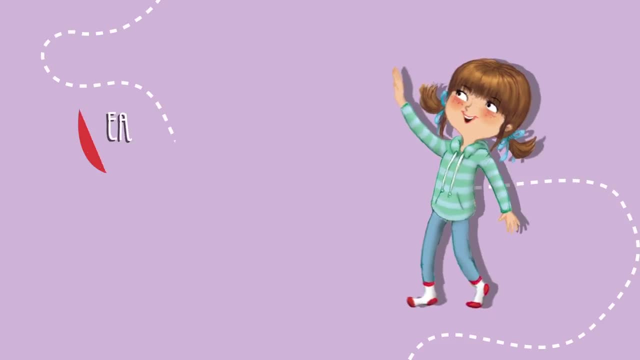 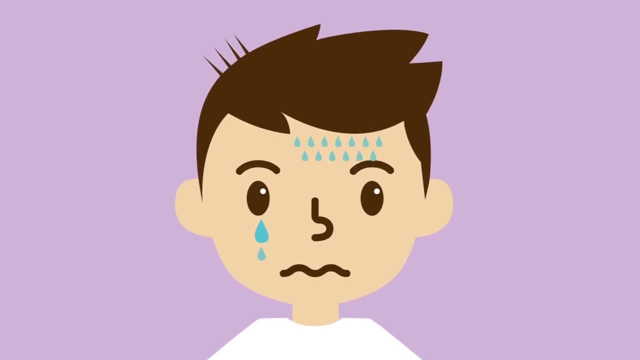 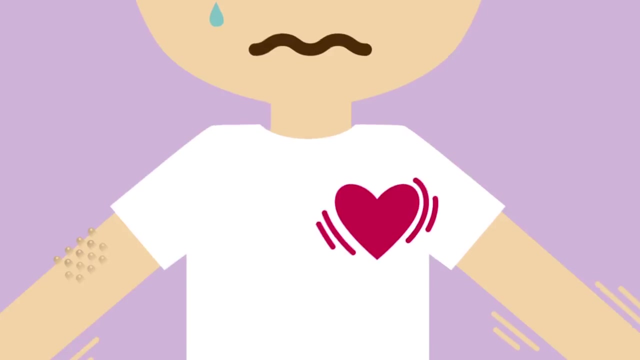 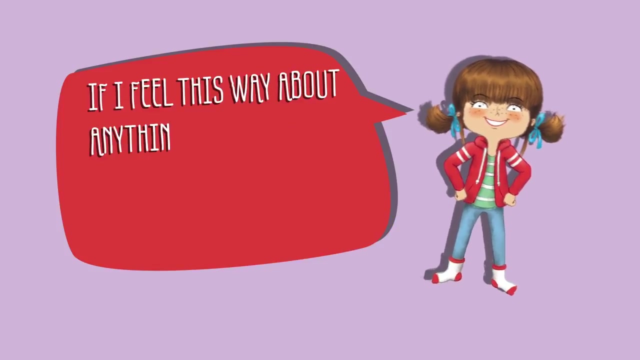 3. Early warning signs. If I feel frightened or unsafe, I may sweat a lot, get a sick tummy, become shaky and my heart might beat really fast. These feelings are called my early warning signs. If I feel this way about anything, I must tell an adult on my safety network straight away. 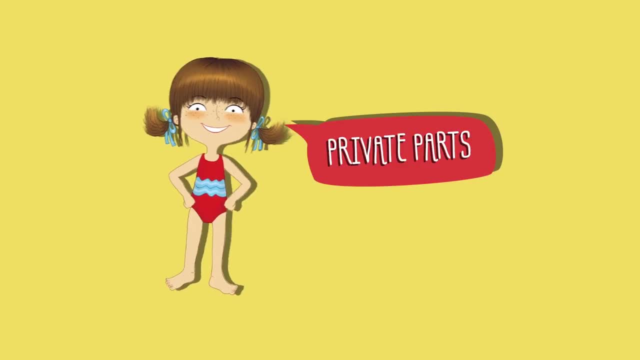 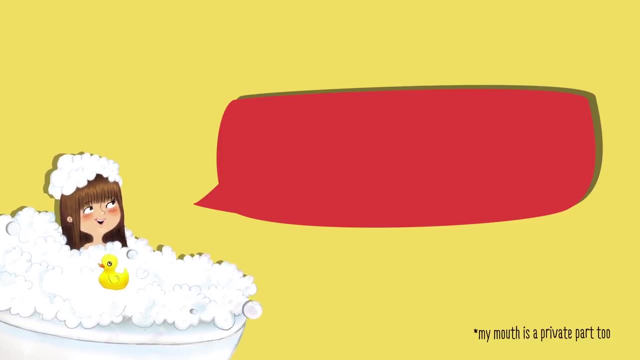 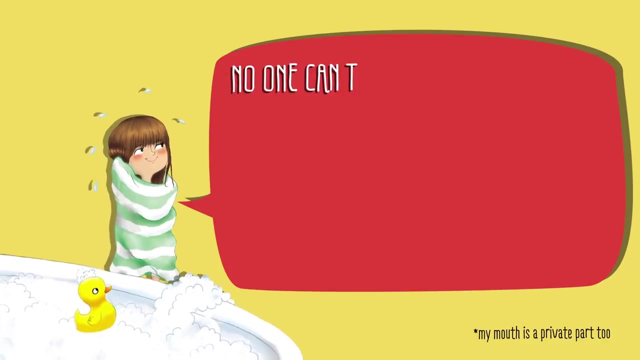 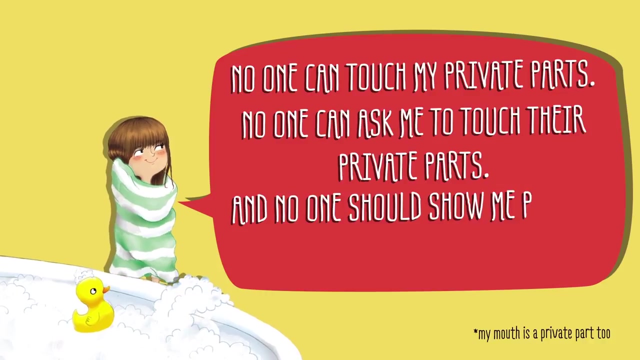 4. Private parts. My private parts are the parts of my body under my bathing suit. I always call my private parts by their correct names. 5. No one can touch my private parts. No one can ask me to touch their private parts And no one should show me pictures of private parts. 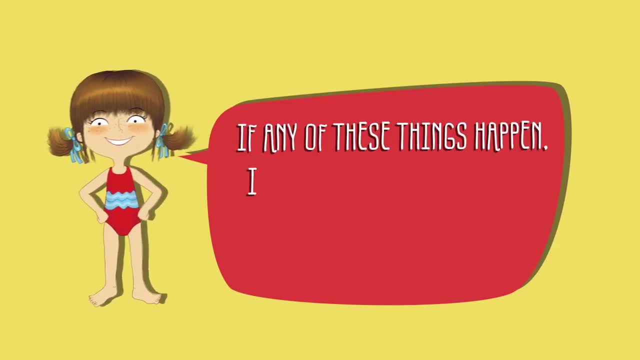 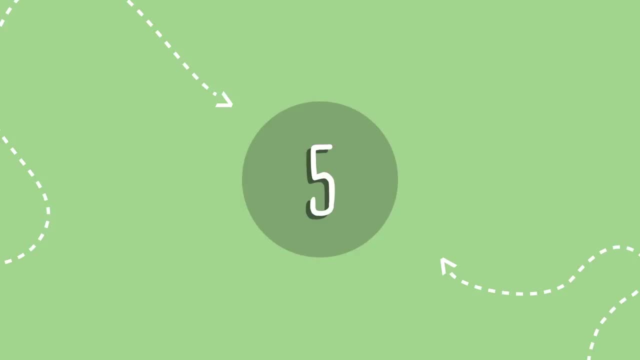 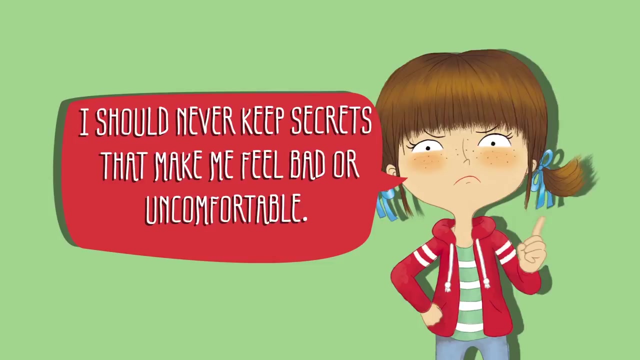 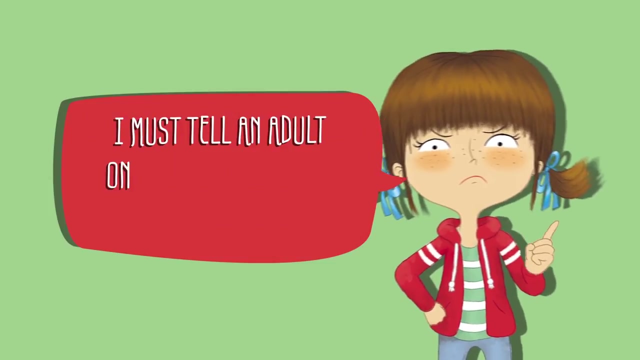 6. If any of these things happen, I must tell a trusted adult on my safety network. 5. Secrets: I should never keep secrets that make me feel bad or uncomfortable. If someone asks me to keep a secret that makes me feel bad or unsafe, I must tell an adult on my safety network straight away. 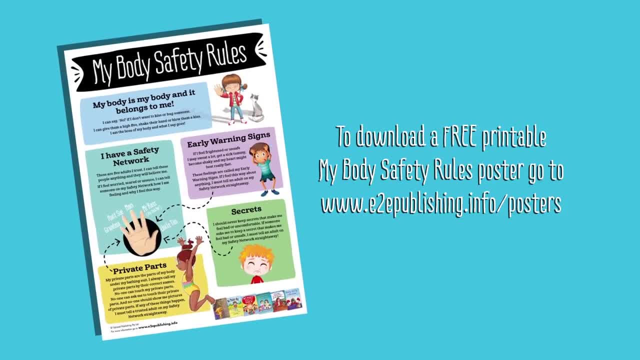 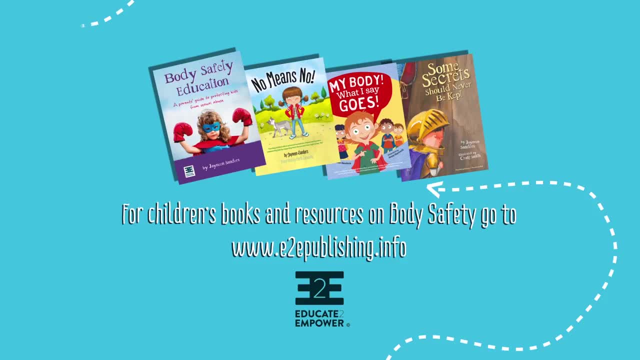 My body is my body and it belongs to me. Thanks for watching.